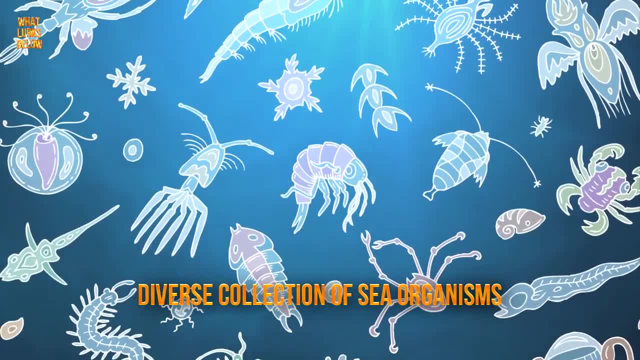 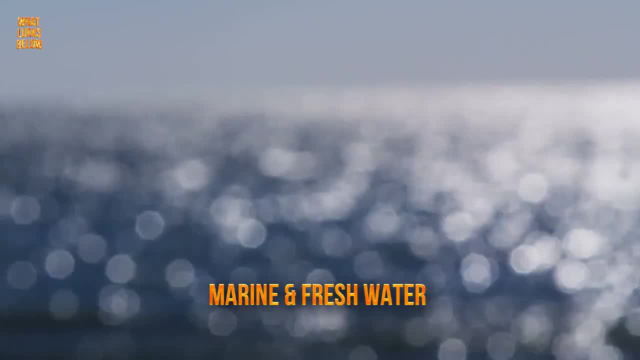 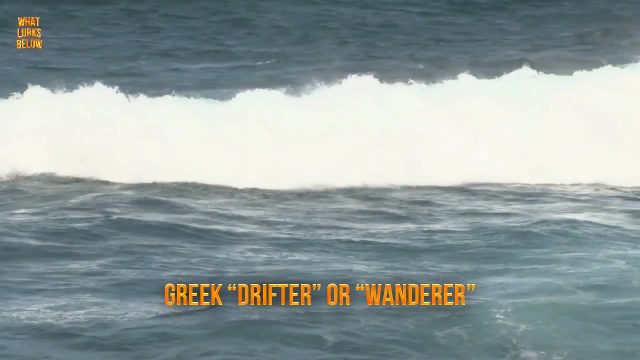 Plankton comprises of a diverse collection of sea organisms that dwell in larger bodies of marine and fresh water. Due to their carefree nature, their name literally translates from Greek to Drifter or Wanderer. While they are so tiny, one must bear in mind that just because you can't see them doesn't 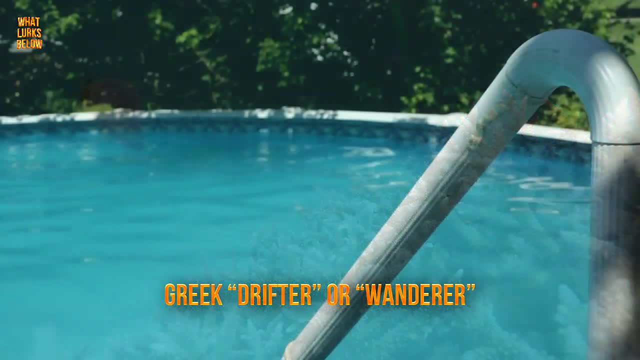 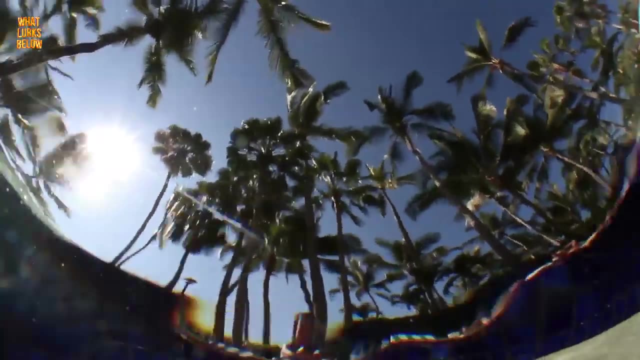 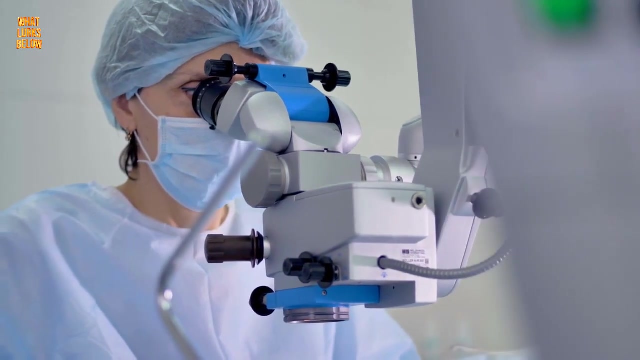 mean that they aren't there. The next time you investigate what appears to be an empty tide pool, know that there are hundreds of microscopic organisms inhibiting that water. While small, these sea drifters are so important That marine phytoplankton has been called single-celled microscopic algae, upon which 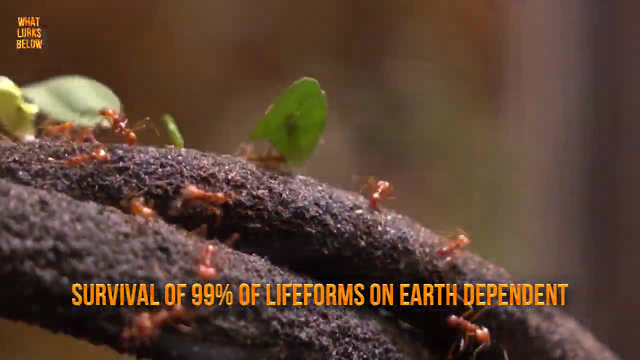 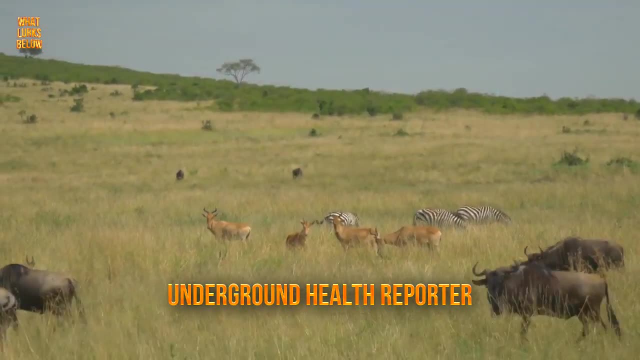 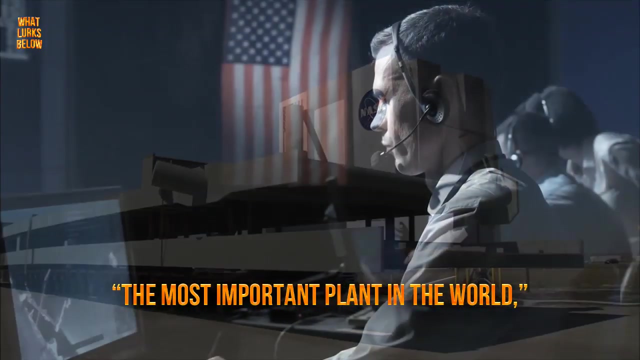 the survival of 99% of all life form on earth depends, according to research from the Underground Health Reporter- And you know you've made it in the world when you receive a shout out from NASA, for the administration deemed you as the most important plant in the world, as they make. 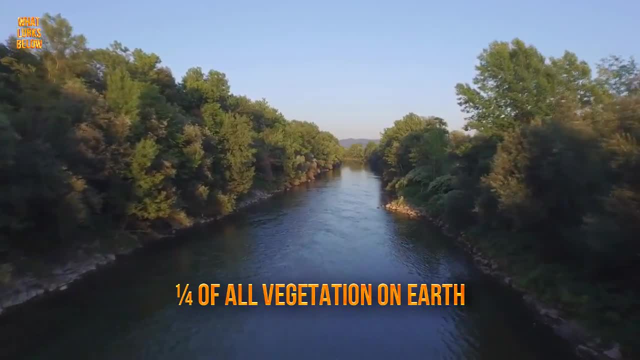 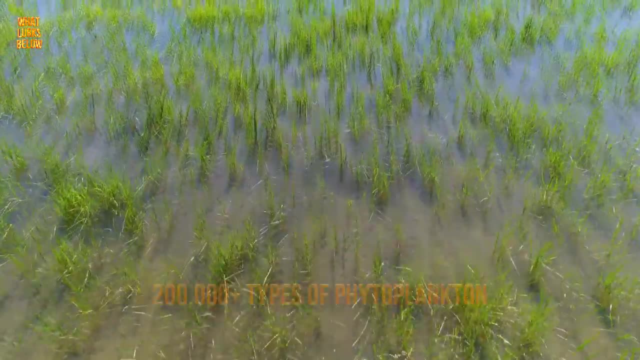 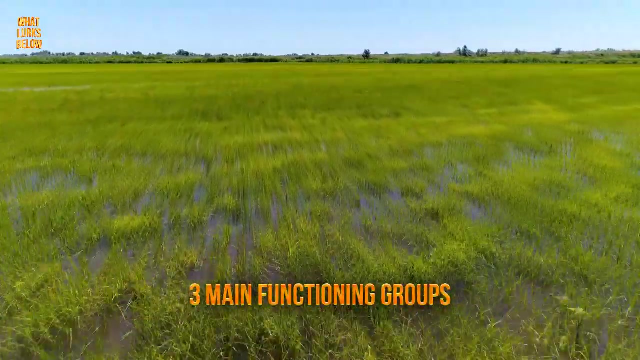 up a quarter of all vegetation on earth. That's a lot for scientists to determine that there is an infinite number of species, due to the fact that there are over 200,000 types of phytoplankton alone. Within this vast class, there exist three main functioning groups: phytoplankton, zooplankton. 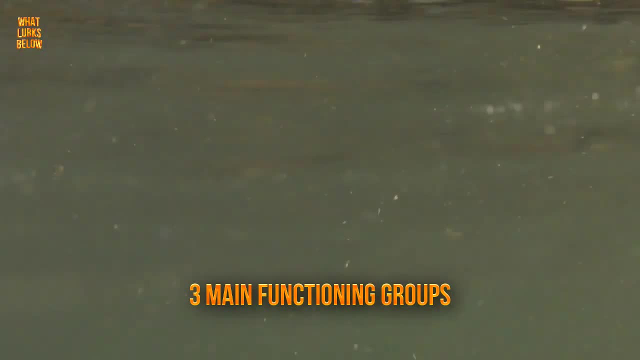 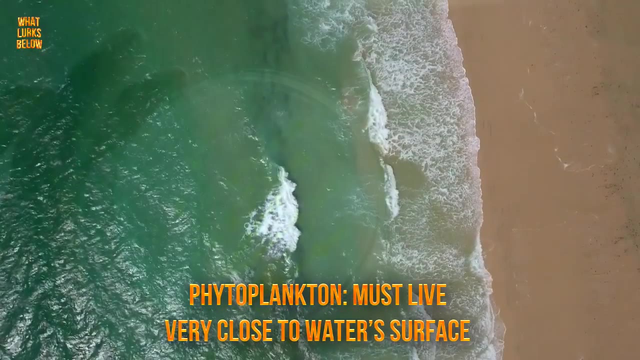 and bacterioplankton. The first is made up of very tiny, usually always single-celled plants. Phytoplankton must live very close to the surface. Phytoplankton must live very close to the surface. Phytoplankton must live very close to the water surface, since they steal the sun's. 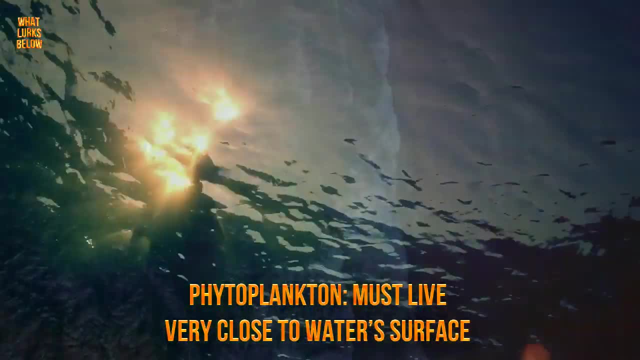 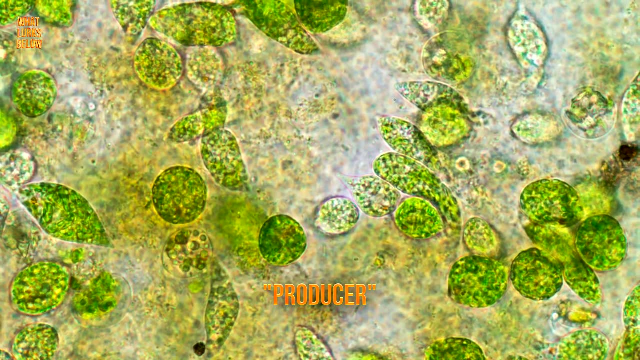 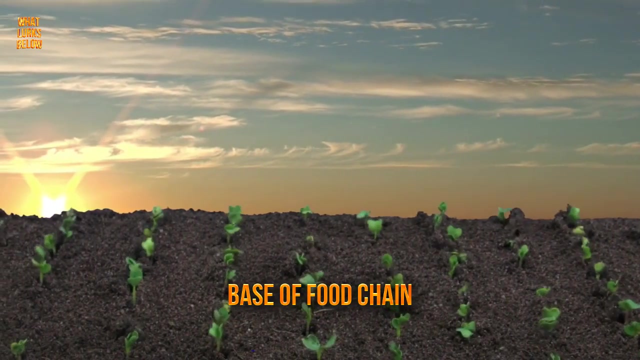 energy to be used in their own process of food production. This method of photosynthesis earns plankton the title of producer, and thus they have been placed, accordingly, at the very base of the food chain. As plants create their own energy and release oxygen as a byproduct, all other marine life 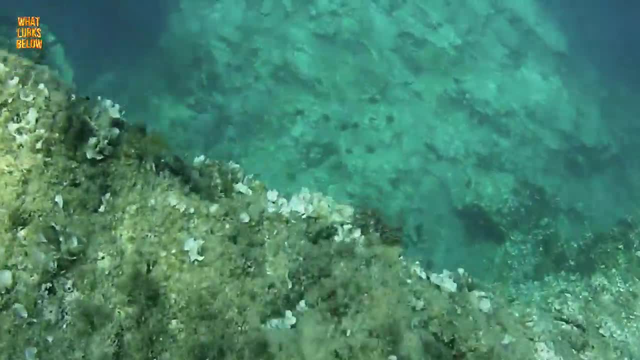 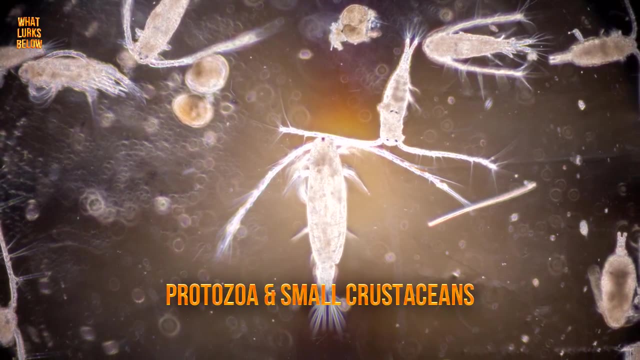 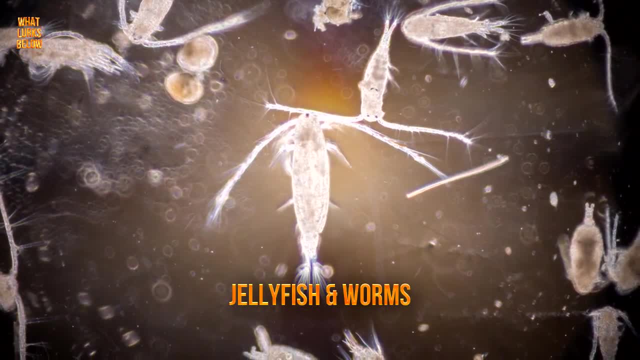 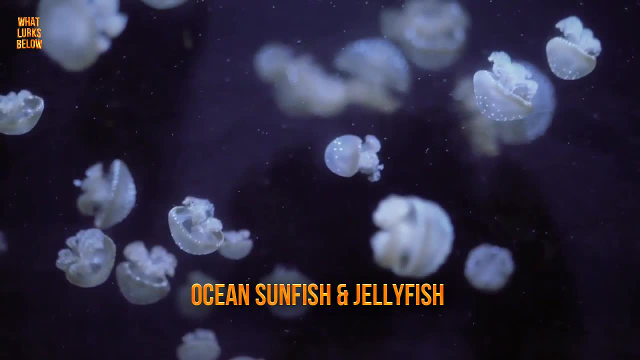 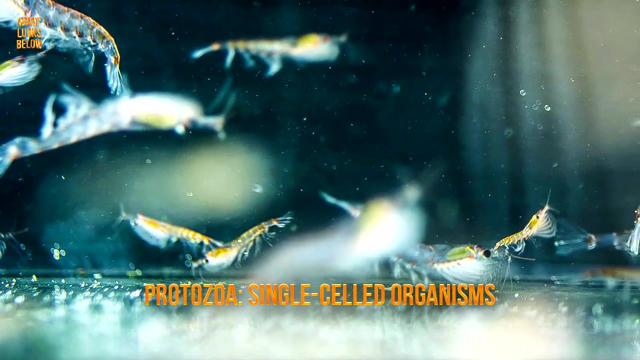 crustaceans, jellyfish and worms. Ocean sunfish and jellyfish fall into this category due to their feeble ability to swim and their nature to drift and flow with the commanding tide. Protozoa are single-celled organisms that like to 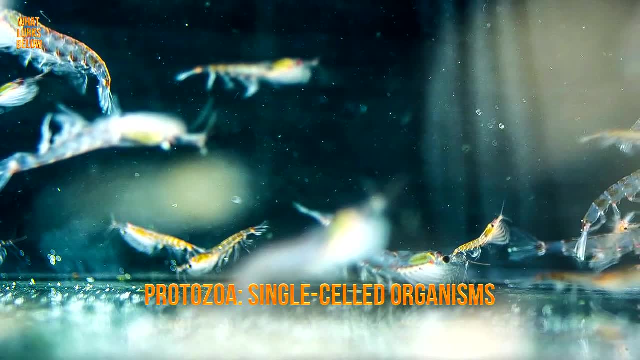 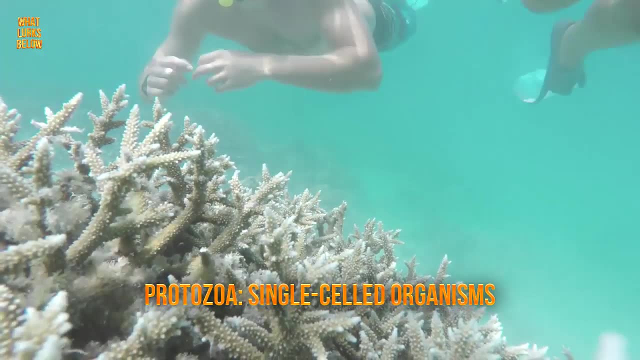 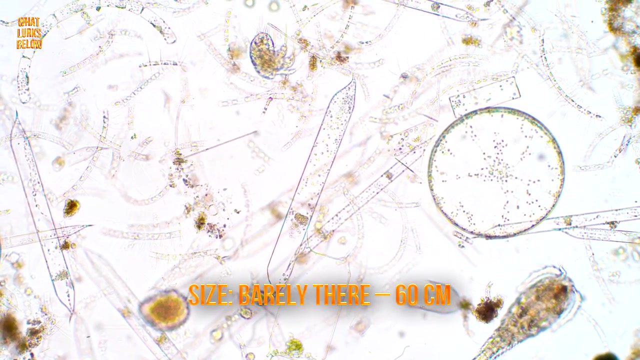 colonize and can vary in size. They can be found in a variety of bodies of water, such as the oceans, salt and freshwater, lakes, rivers and ponds. Crustaceans are invertebrates that live in both water and on land and can range in proportions. 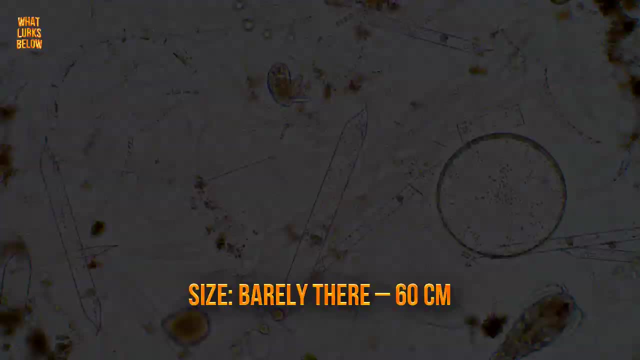 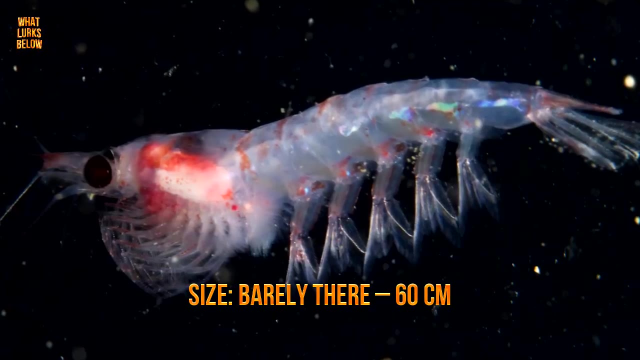 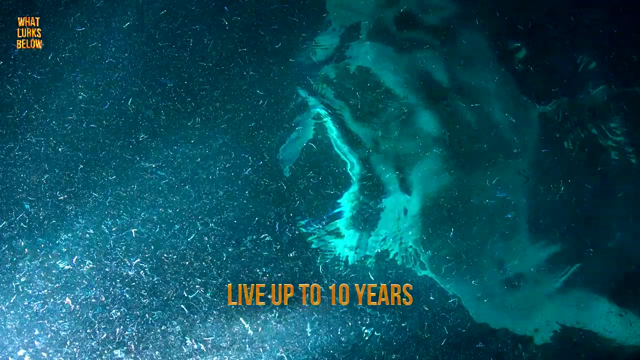 from barely there to 60 centimeters. Their tiny counterpart, krill, contains swarms of small organisms belonging to the crustacean species. These guys are cool in themselves as, despite being one of the ocean's most heavily hunted, they can live up to 10 years by avoiding predators amid murky depths up to 320. 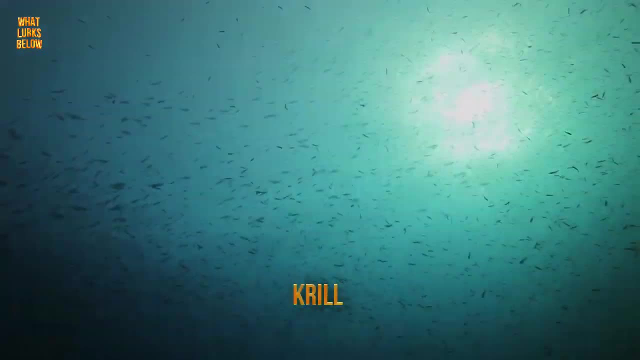 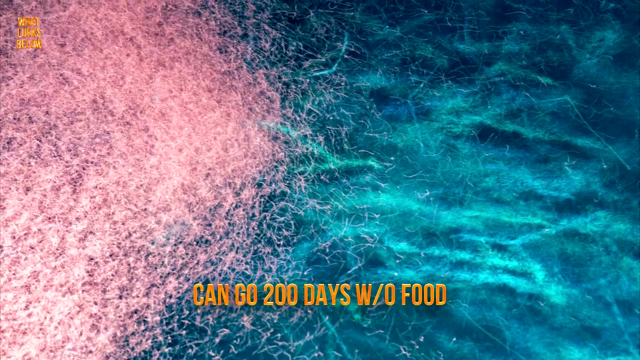 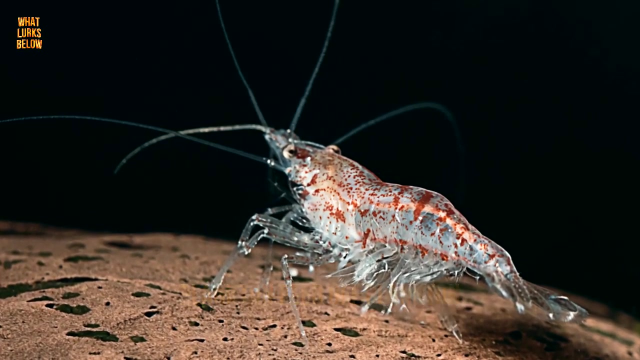 feet and in cold depths of the Antarctic. Krill can go up to 200 days without the consumption of food and, in accordance with any extreme diet, will shrink in size so that they survive. The life cycle of plankton is so generous that even plankton feeds off of the crustacean species. Protozoa are also known for their 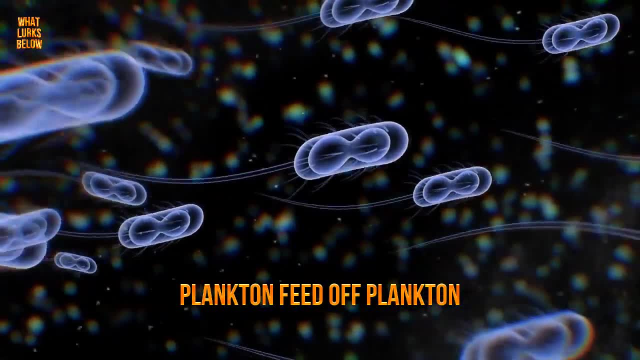 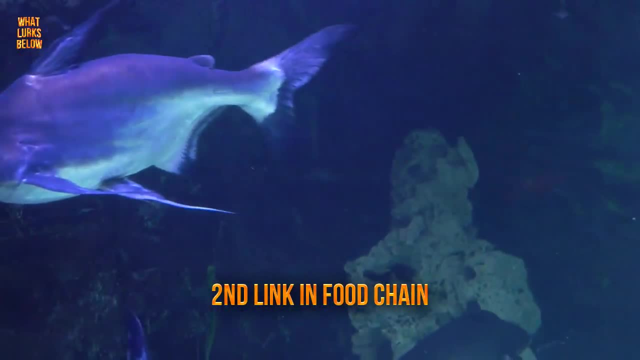 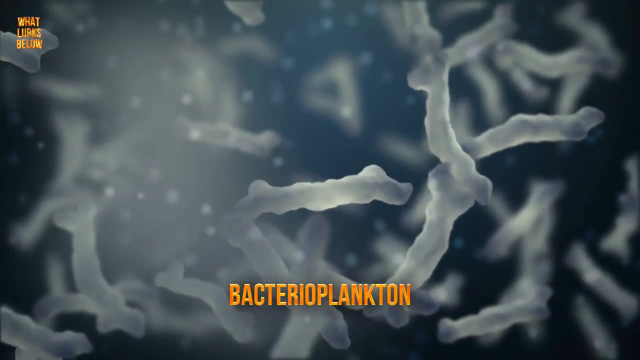 growth of plankton. For zooplankton, their primary sustenance stems from bacteria and phytoplankton, which makes them the second link in the food chain. Lastly, there is bacterioplankton, referring to the bacteria element of plankton, which shifts seamlessly among the sea's. 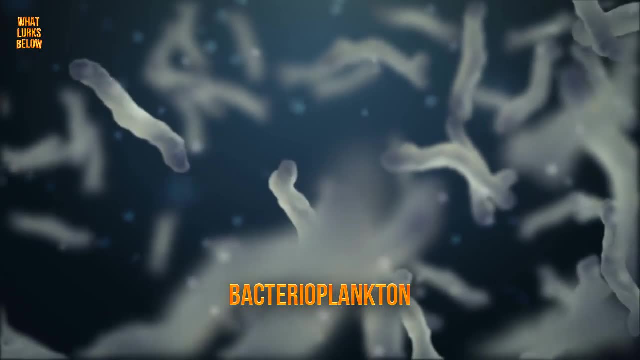 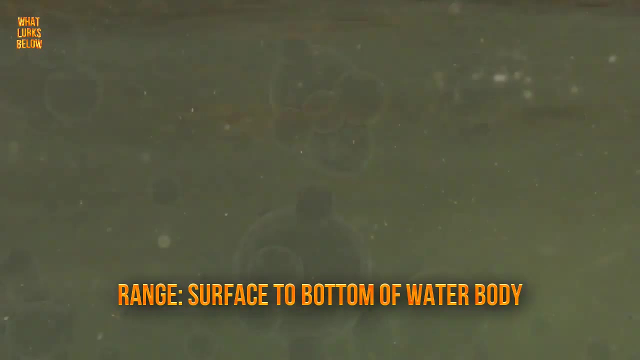 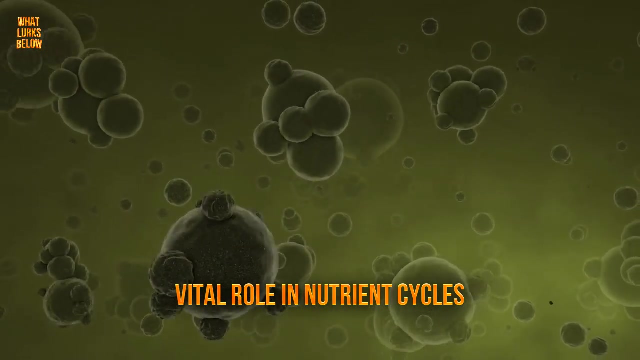 water column, That is, a conceptional column of water ranging from the surface all the way down to the bottom sediment of the ocean, lake or river floor. These little motes of bacteria play a vital role in the nutrition cycles found here. Ultimately, then, 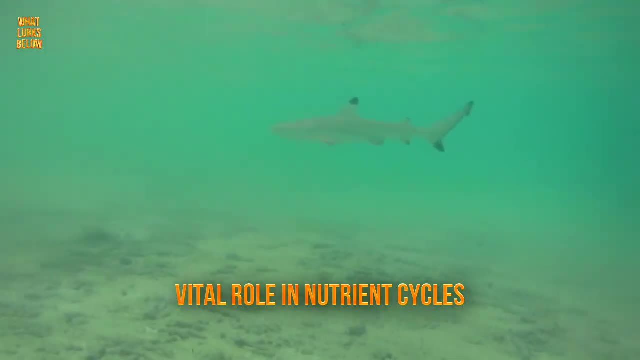 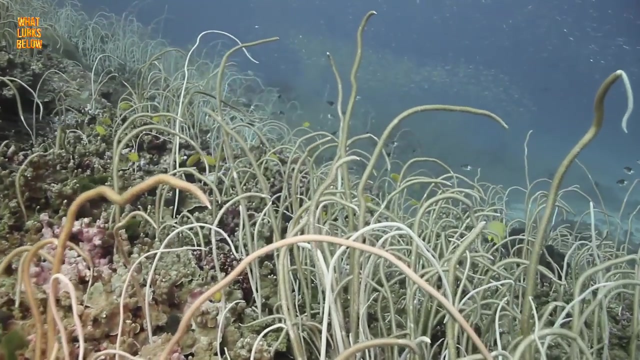 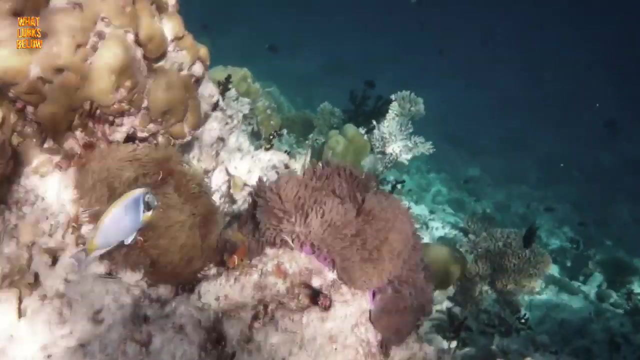 plankton acts as the sole supplier of the upper echelons of the food chain, even feeding humans and whales. Since most of the plankton in the ocean are plants, they are a go-to snack for most animals and those who don't opt for these protein-packed, bite-sized morsels. 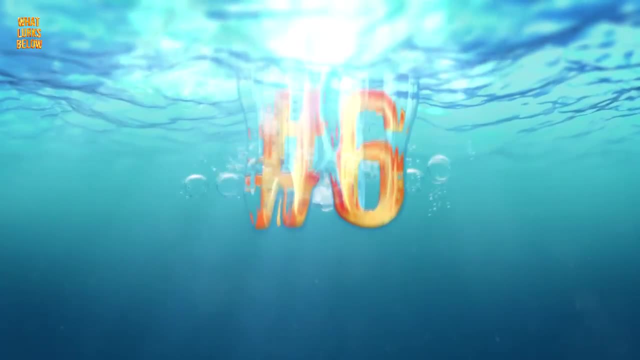 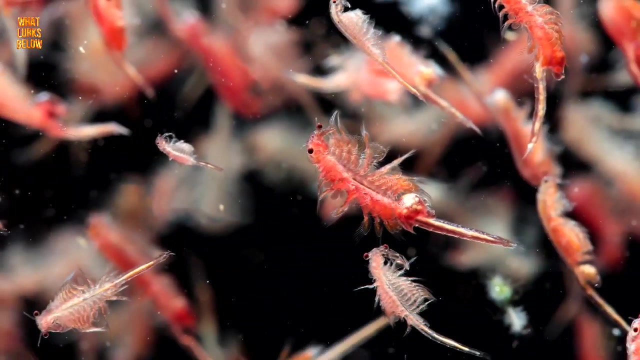 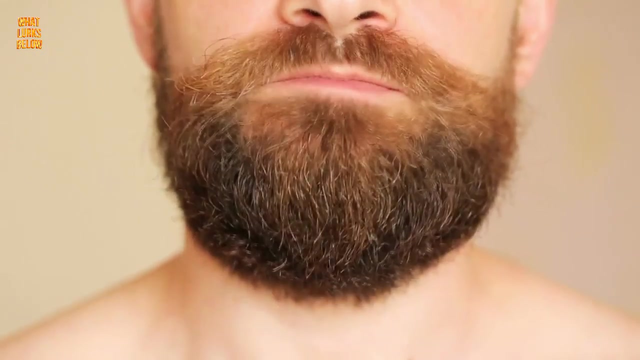 feast on creatures which do. Number 6 – You Are What You Eat. Maybe we can't all be sunshine yet. plankton are such a superfood, chock full of nutrients that munching on these little guys may very well be the equivalent to chowing down on golden. 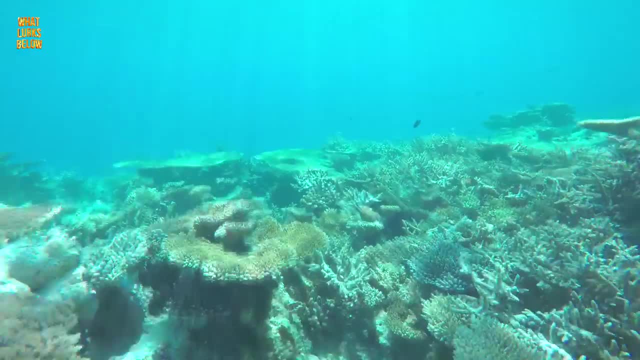 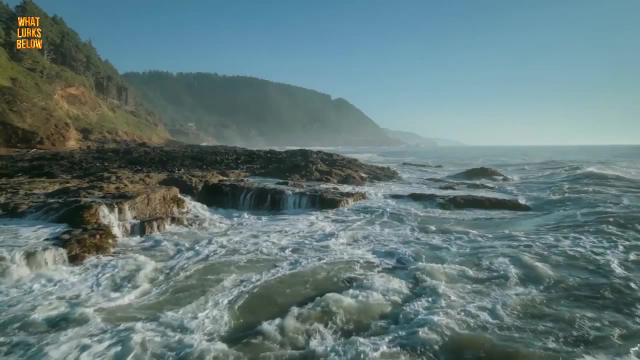 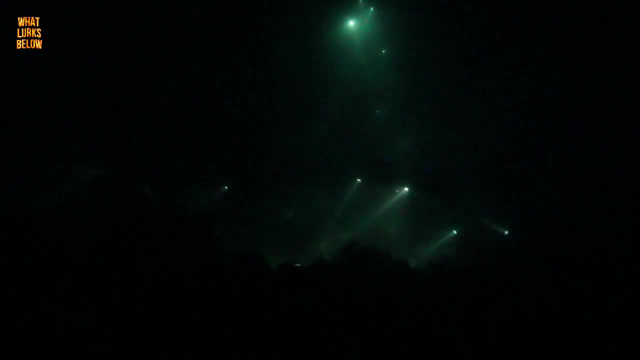 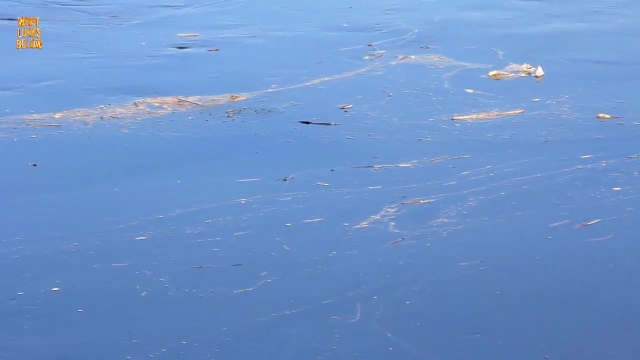 proverbial bottom of the food chain. when you're all the way down, way down, there's nowhere left to go but up, way up. Phytoplankton flourish on the water's surface where it can rope in the sun's effervescence. 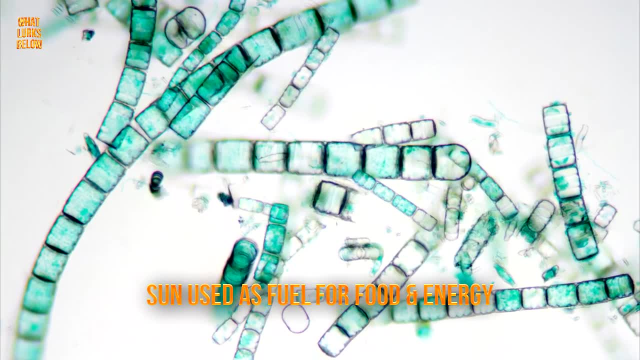 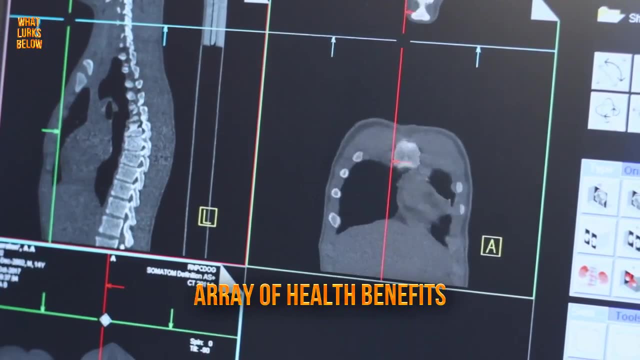 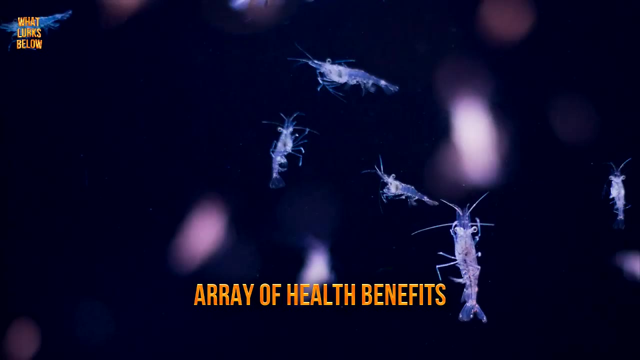 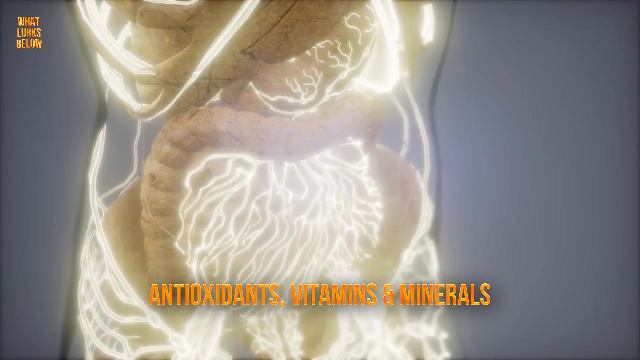 to use as fuel for food and energy, Due to this, phytoplankton are robust superfoods which boast an array of health benefits And, in a society where food trends are all the rage, health enthusiasts have flocked to this one, For plankton. contain a ton of amino acids, healthy fats, antioxidants, vitamins and minerals. 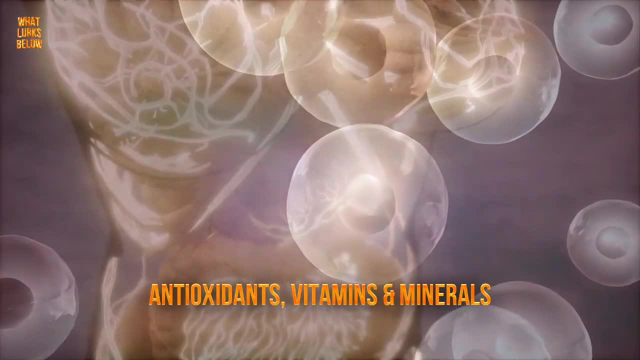 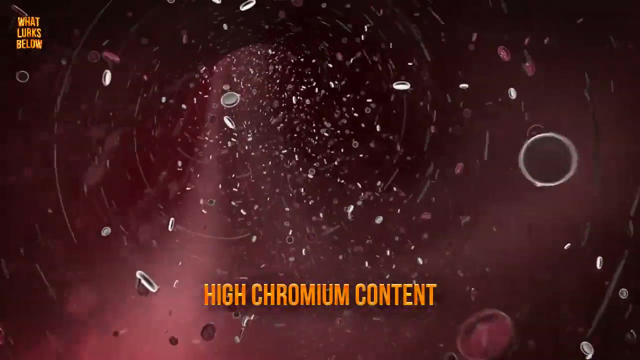 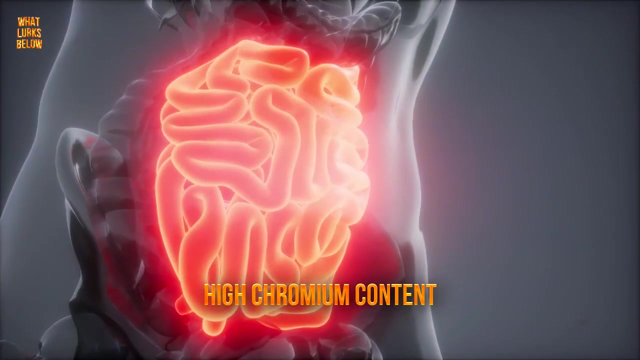 that support the body all the way down to the cellular level. In addition, phytoplankton helps balance blood sugar, Due to plankton's high chromium content. consumption then meddles with blood sugar regulation to help insulin. In addition, phytoplankton can help insulin move glucose that can be burned as energy. 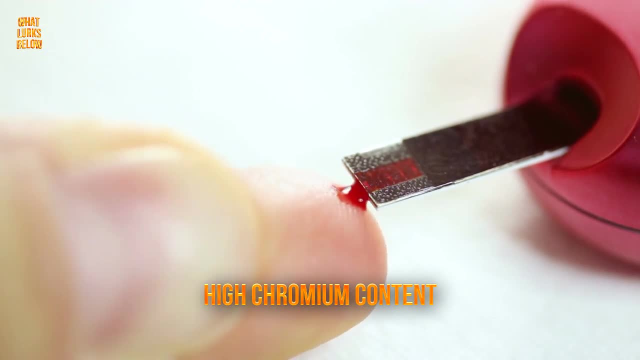 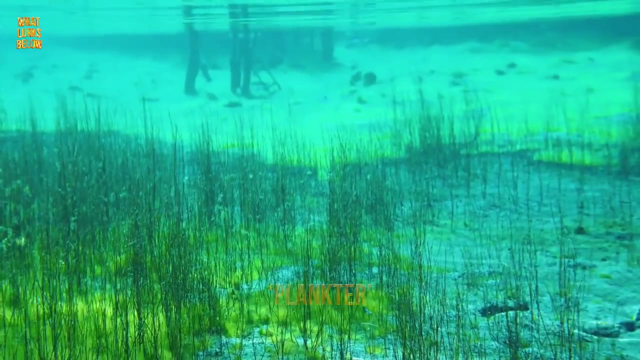 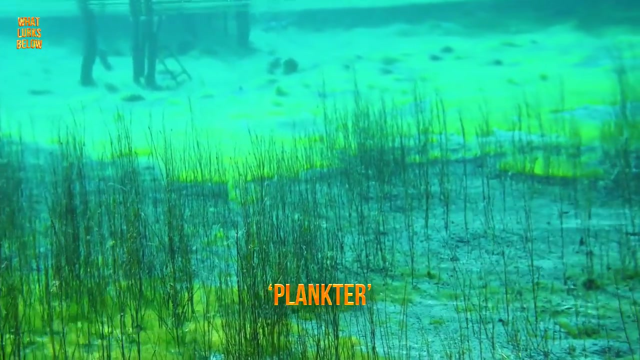 This is especially important for those who suffer from diabetes or who are pre-diabetic. Number 5, They are a Natural Cleanser. Plankton, or plankters as they are called in their individual form, lead a seamless life of leisure simply by going with the flow. 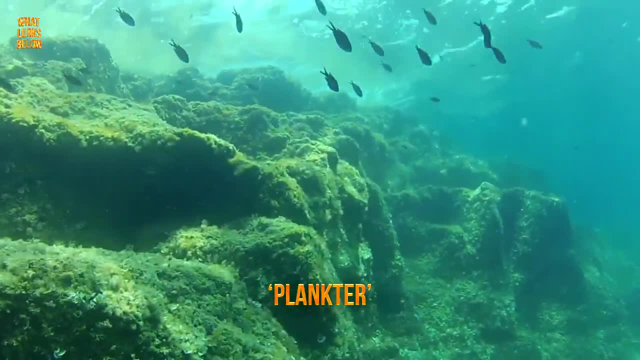 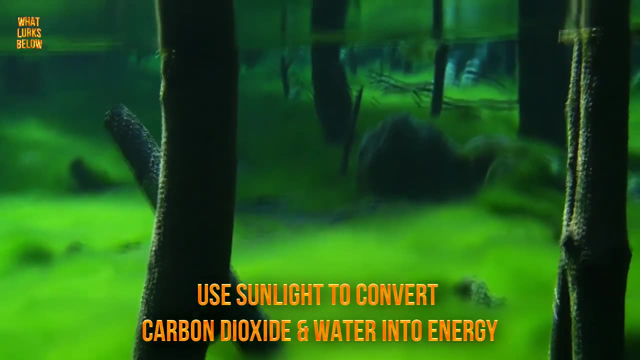 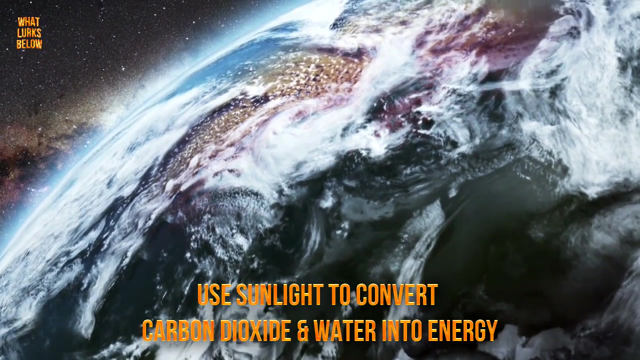 At least it would appear so. Phytoplankton's natural organisms are hard at work, making our lives as easy as breathing. That's because phytoplankton use sunlight to convert carbon dioxide and water into energy at an astonishing rate. In turn, these efforts help regulate CO2 levels in the atmosphere. 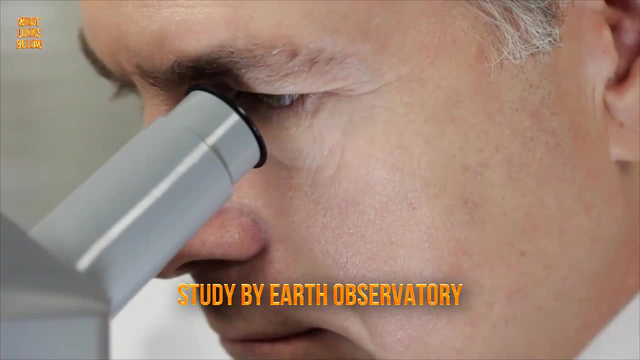 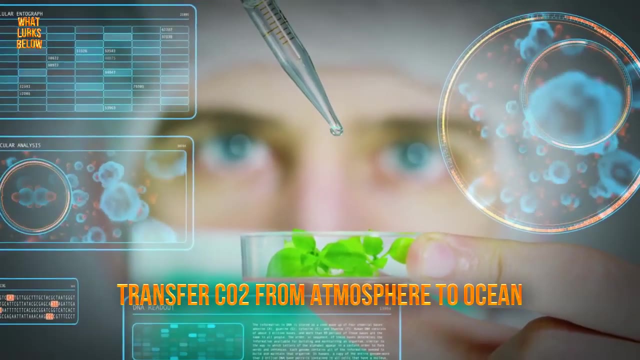 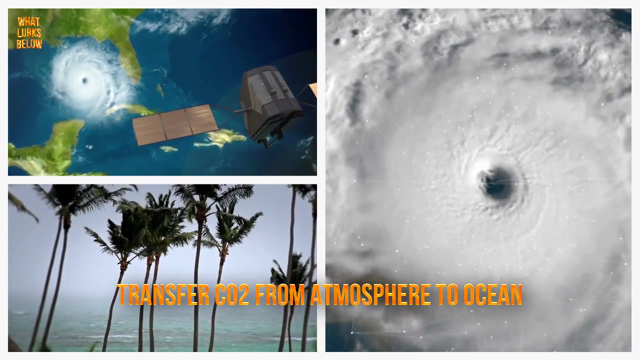 In a study by Earth Observatory, scientists determined that phytoplankton are responsible for a large amount of transfer. In fact, phytoplankton are responsible for a large amount of transfer of CO2 from our atmosphere to the ocean. Given the severe authority of carbon dioxide on the side effects of climate change, phytoplankton 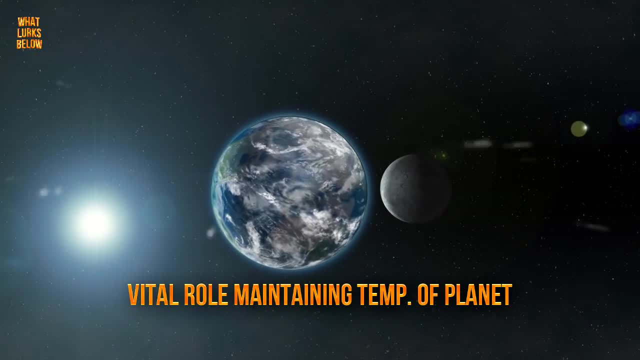 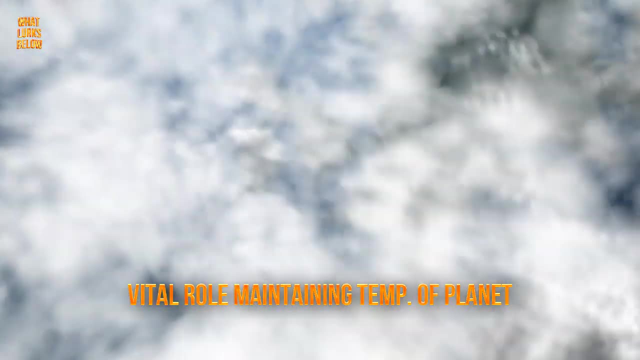 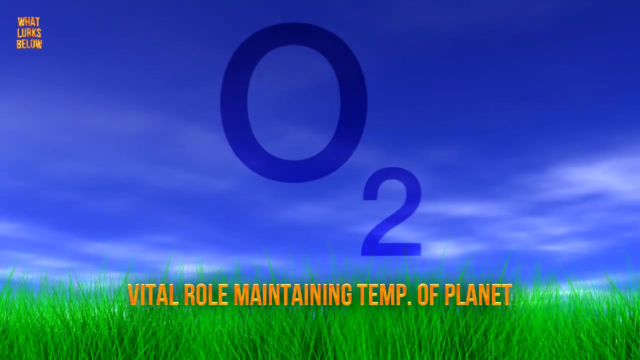 play a vital role in maintaining the temperature of the planet and keeping it under wraps. The more CO2 chokes the atmosphere, the quicker plankton can convert these chemicals into clean air. Ultimately, the conversion of carbon into oxygen greatly decreases the amount of carbon. 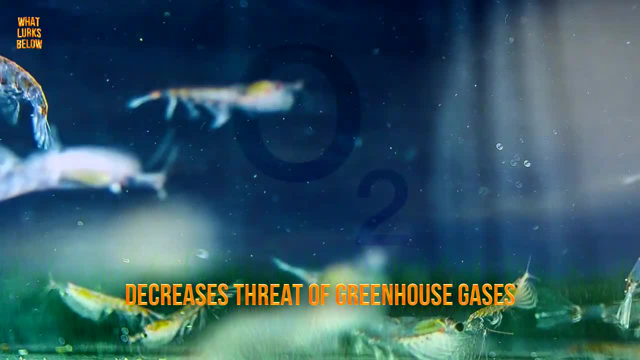 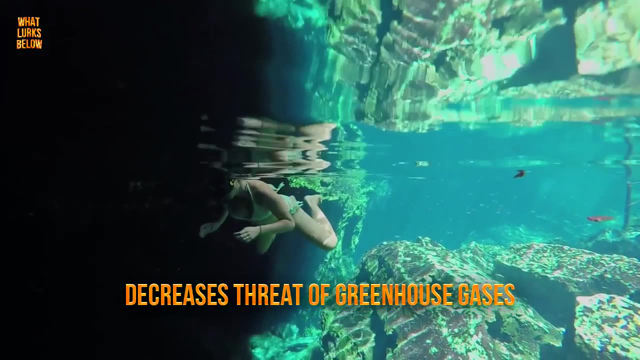 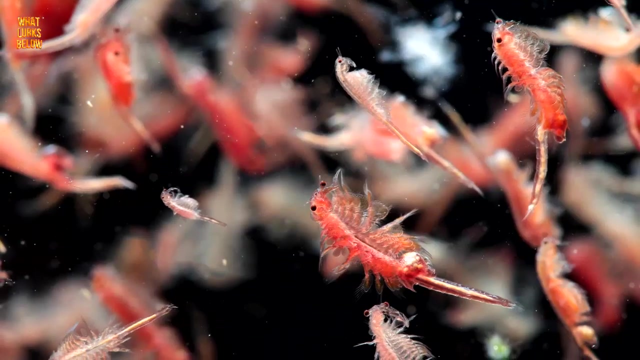 dioxide in the atmosphere and increases the threat of greenhouse gases. So, while these creatures may seem like simple chilled out critters of the open sea, their existence plays a vital role in helping others. Number 4, They're No Wimp. Speaking of plankton as a popular delicacy among the 200,000 species of phytoplankton, 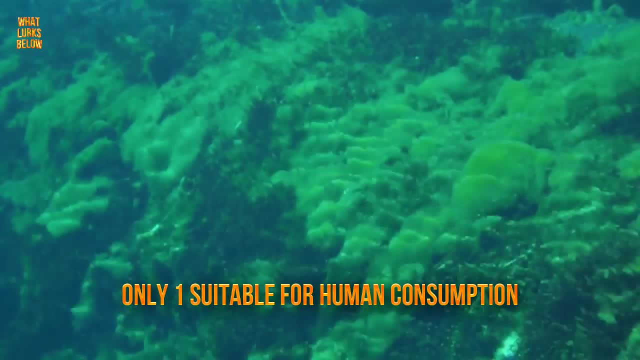 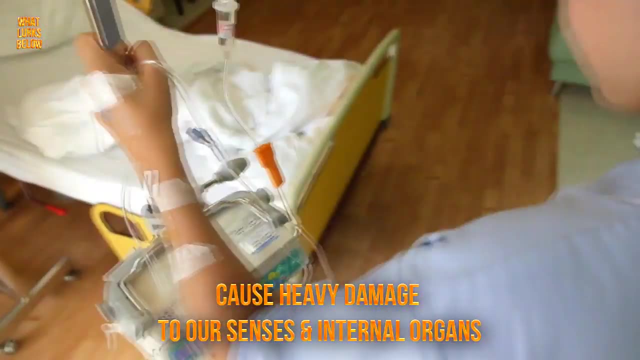 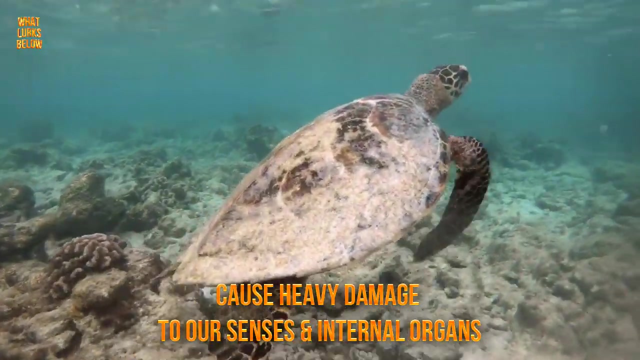 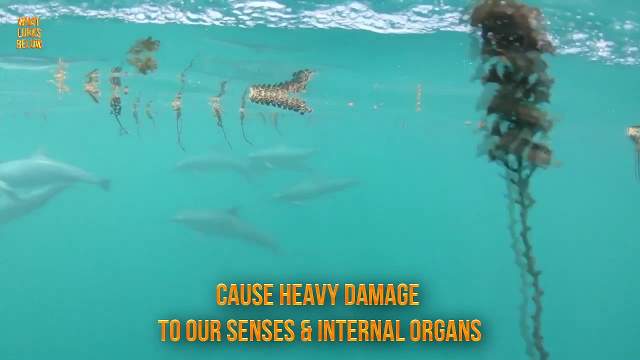 alone, only one type is suitable for human consumption. This means that almost all of plankton possess characteristics that can cause heavy damage to our senses and internal organs. While phytoplankton has proved safe for animals, the following species produce harsh chemicals and poisons that can make a person very sick. 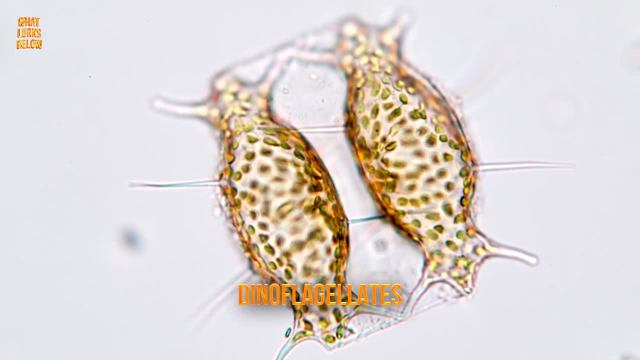 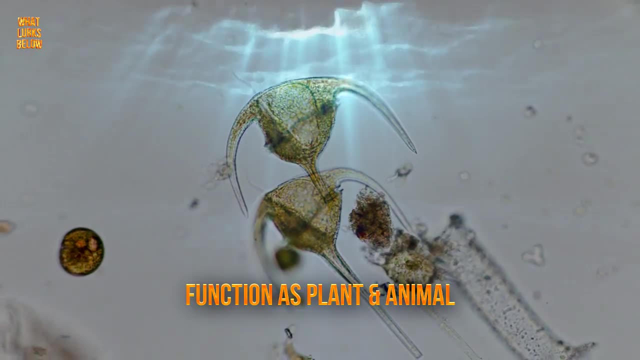 Dinoflagellates they're called, and they exhibit the capability to function as both plant and animal. This member of the phytoplankton family can become a very dangerous parasite. Number 5, Dinoflagellates. This member of the phytoplankton family can move through water using the grooves placed. 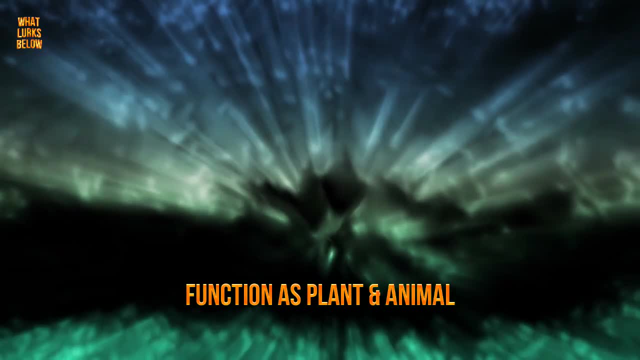 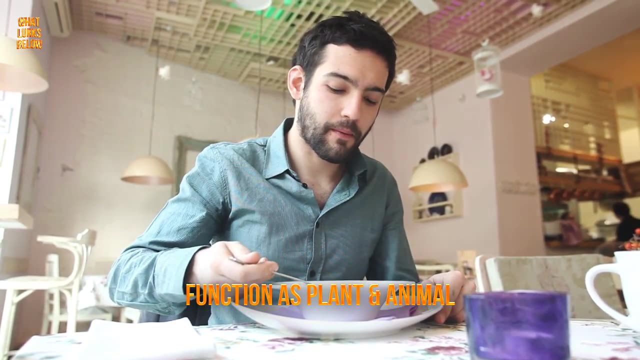 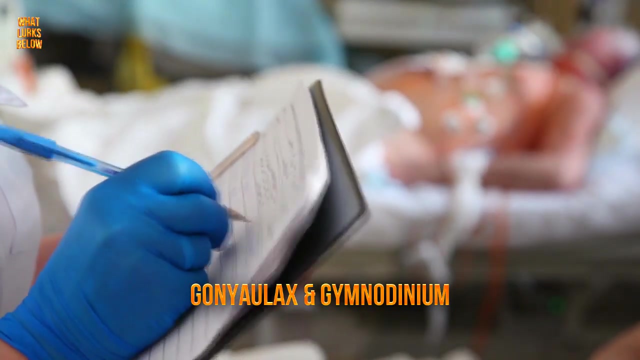 along their body, while also utilizing photosynthesis to produce food, as plants do. Human digestion of the two species of dinoflagellates, Gonulix and Gymnodynium, lead to uncontrollable bowel movements, paralysis, dizziness and long-term memory loss. 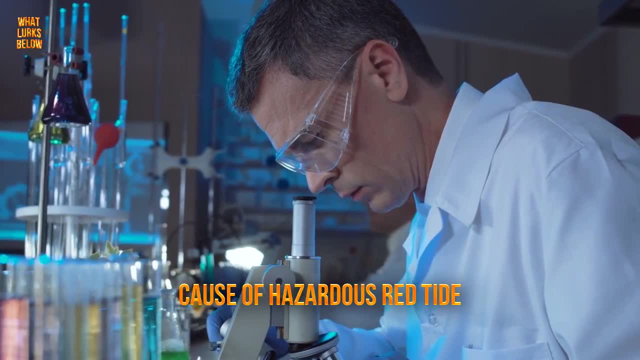 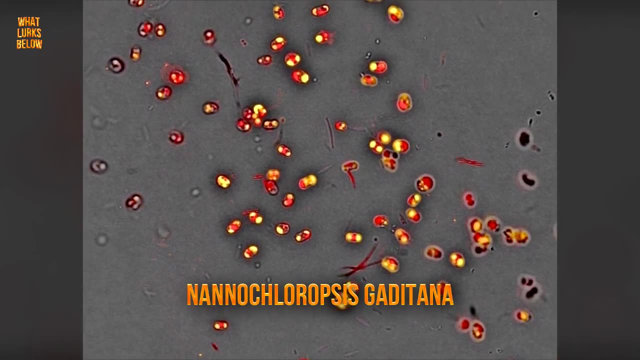 This toxic duo is also the cause of hazardous red tide Number 6, Red Tide. In this case, size matters. One strain of marine phytoplankton, Nanochloropsis ganitana, to be put simply, is so tiny in dimension. 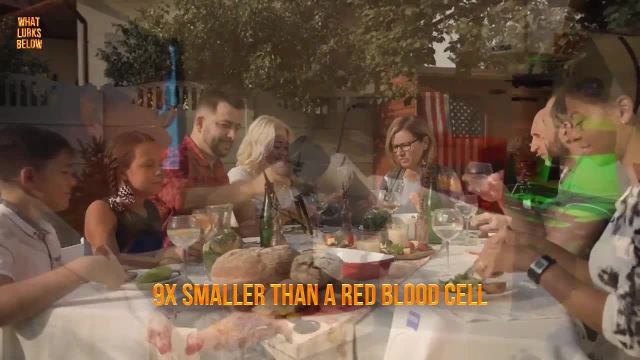 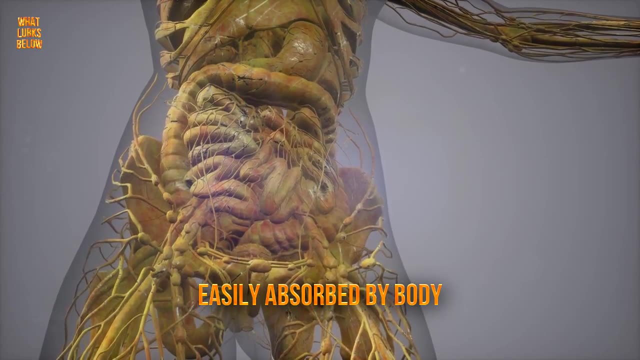 it is nine times smaller than a red blood cell. This makes the superfood so easily absorbed by the body that it swiftly provides the immune system with the necessary nutrients. Also, eating plankton is good for the environment. Sources say that incorporating plankton in our diet is good for our health. 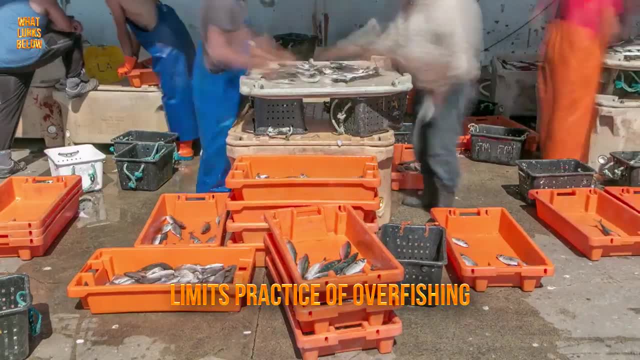 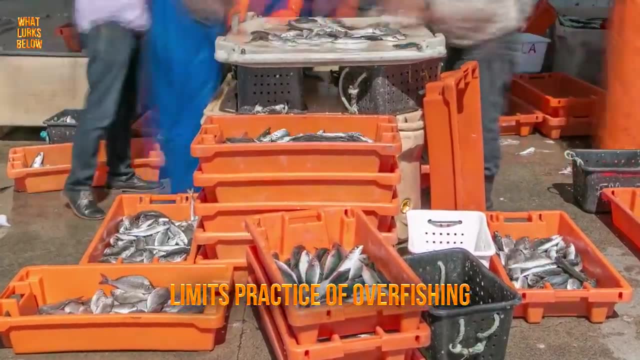 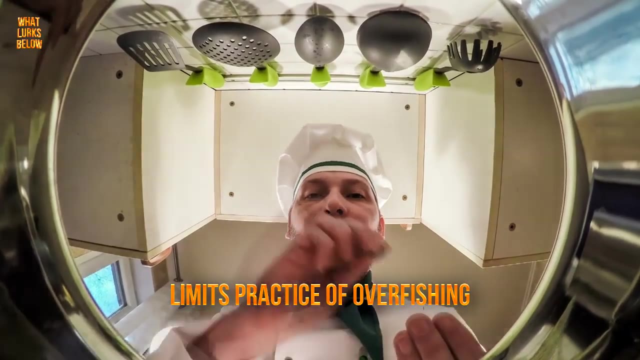 In fact, eating plankton is good for the environment. Plankton in our diets helps limit the practice of overfishing, a critical issue that has chefs engaging in awareness campaigns worldwide. One ocean obsessed culinary guru from Spain is renowned for bringing plankton to the plate. 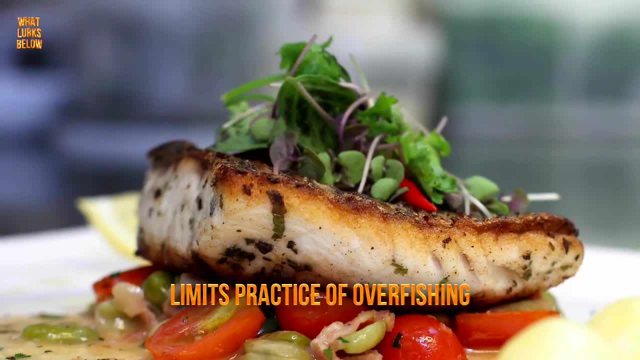 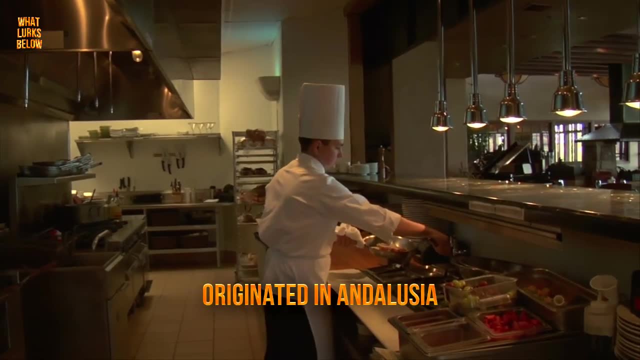 and he makes it glow A staple on his menu. green sea garlic, which has become the world's most popular plankton based recipe. Having originated in Andalusia, Plankton is one of the world's most popular plankton based recipes. 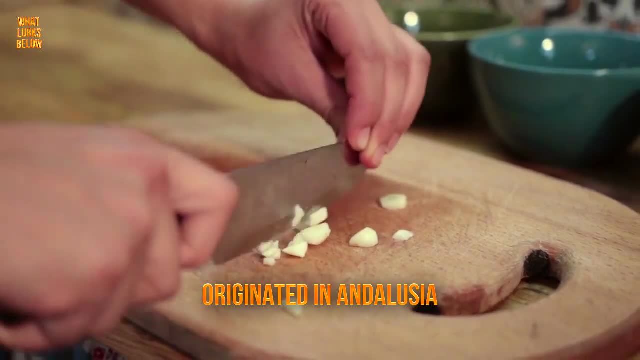 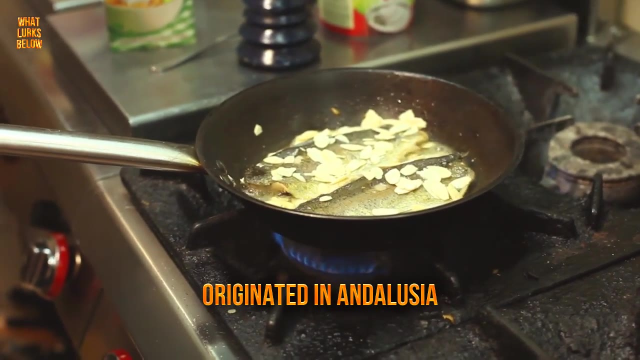 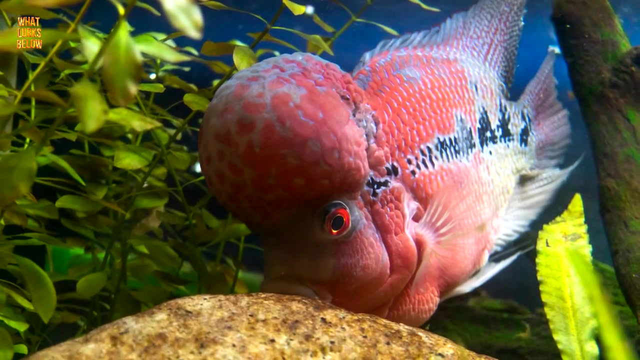 The dish consists of blending almonds, bread and garlic with delicious seed oil. Thanks to the recent innovations in the kitchen regarding plankton, the bottom of the food chain organism is swiftly moving up in the culinary world. The single-celled snack doesn't solely provide sustenance to fish and whales, but now humans. 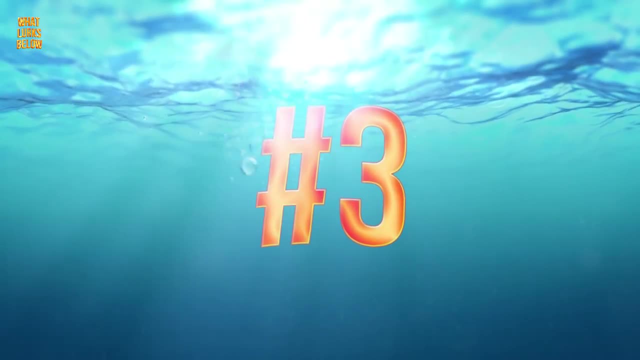 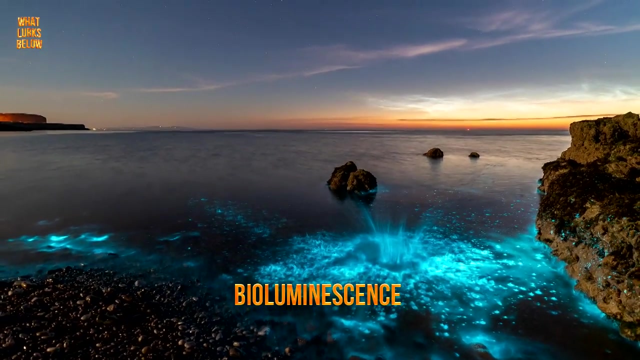 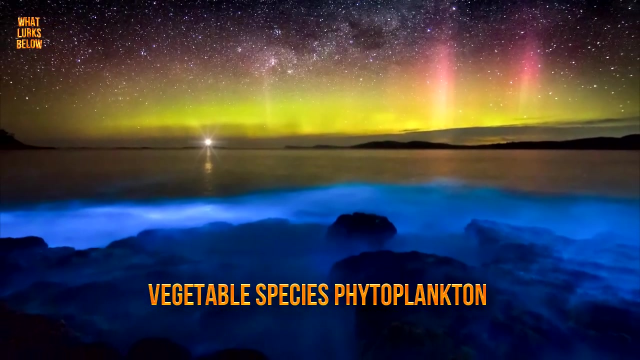 too. Number 3, they look cool To one of nature's aquatic wonders. Plankton is one of the world's most popular plankton based recipes. Look no further than the art of bioluminescence. The vegetable species phytoplankton possesses the ability to emanate a nocturnal glow that 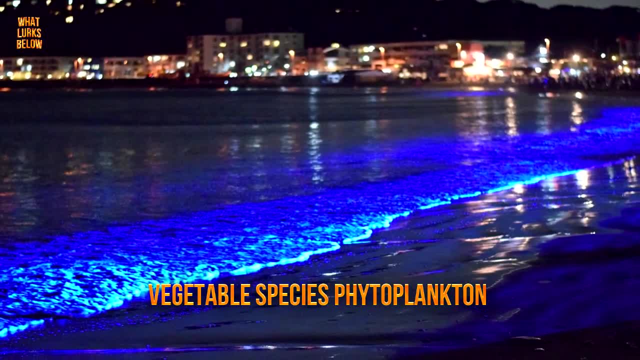 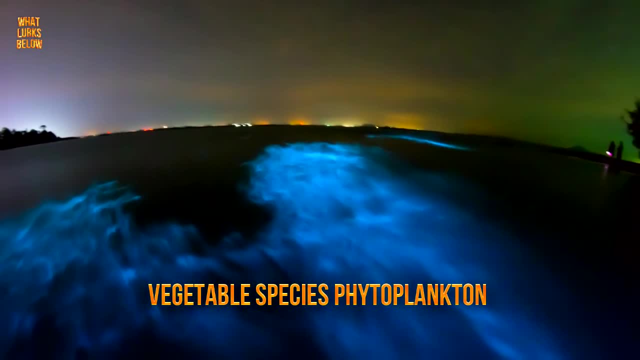 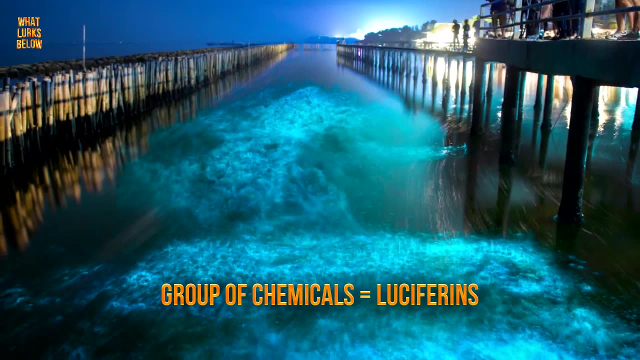 tinges the sea and shades of electric blue. This natural emission is called bioluminescence and can transform the beach by magically igniting the dark waves with profound color Through a group of chemicals called luciferins. light is produced by a series of oxygens and 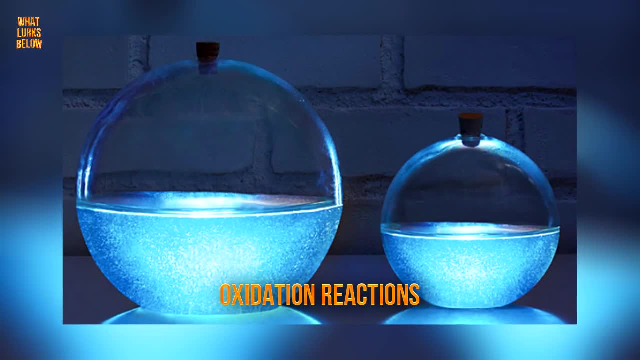 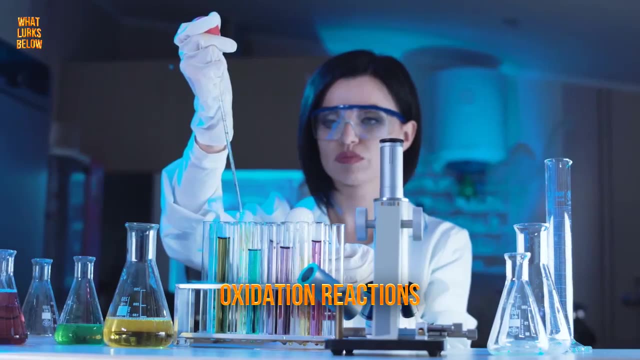 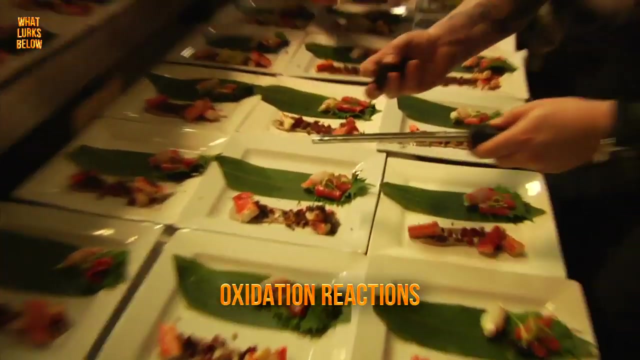 oxidating reactions that in turn make plankton glow. The skill set is prevalent in several forms of the plankton species, and chefs and mixologists have pounced on the pretty sight to use in their own creations. The effect has been exploited with chefs who garnish their plates, as well as bartenders. 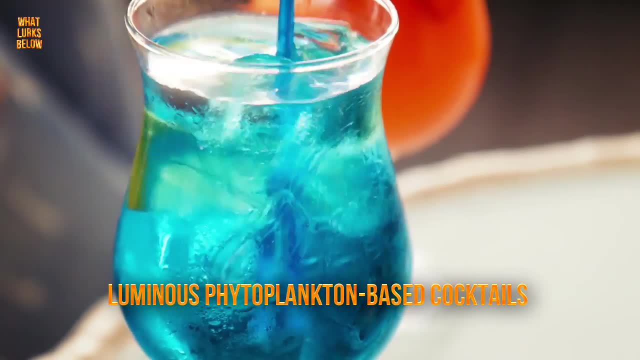 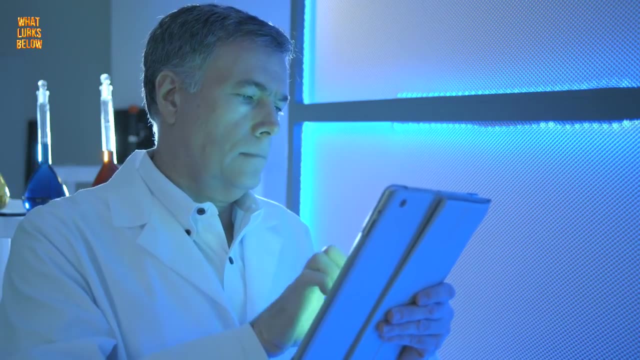 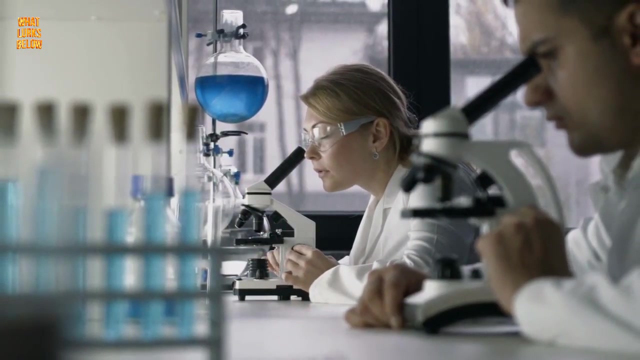 who create luminescent phytoplankton based cocktails- Number 2. They can be used for biofuel. In recent years, researchers have dedicated hours of study to determine the potential of various microalgae species, such as plankton, to be used in the production of biofuel. 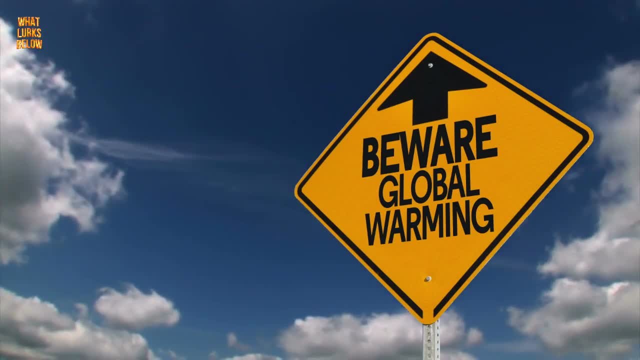 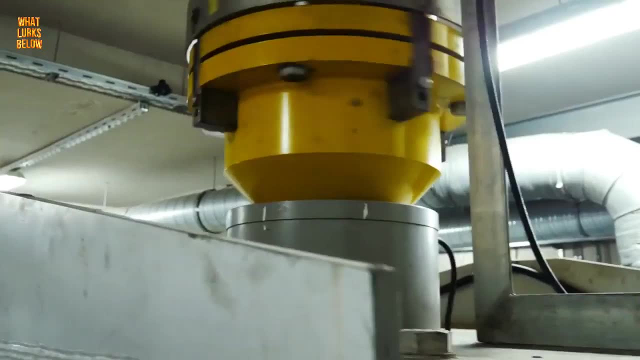 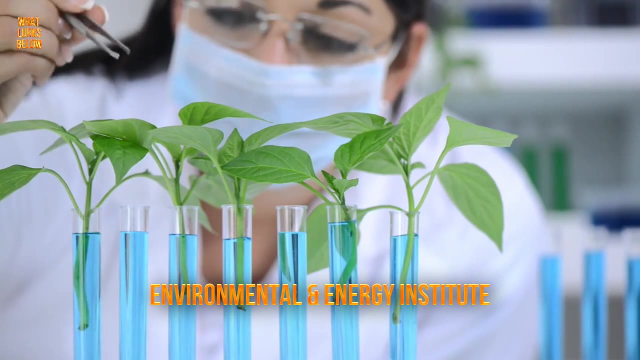 With the impending hazards of global warming a harsh reality in our world today, the environmental impacts of fossil fuels can no longer be denied. The solution: Cleaner fuels that are renewable. According to recent findings at the Environmental and Energy Institute, a marine microalgae 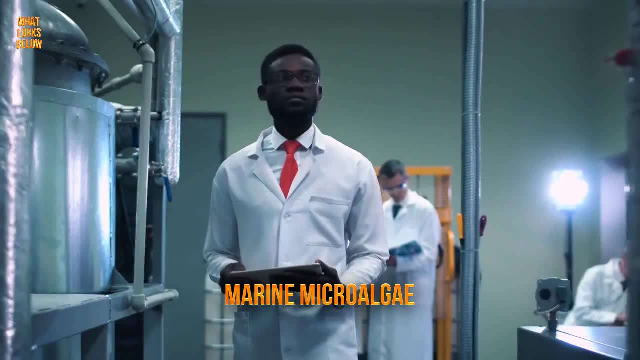 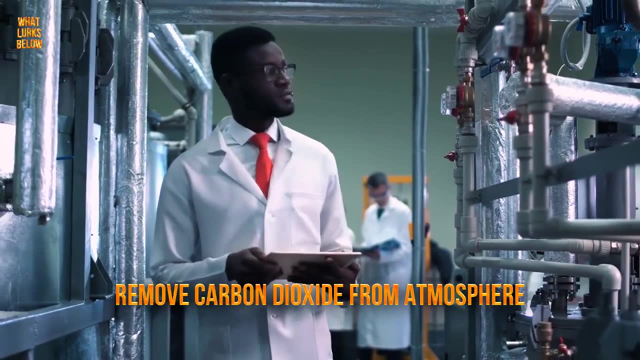 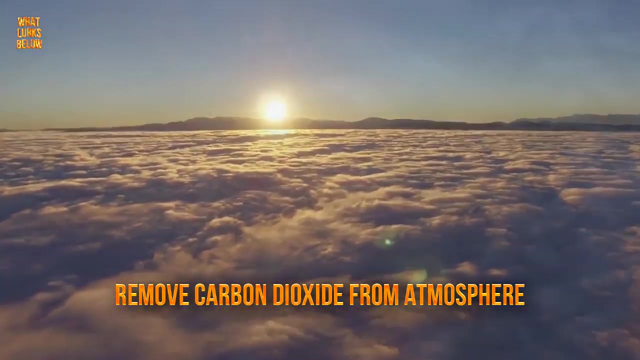 render two very important potentials. First, they possess the mechanisms for carbon sequestration, That is, they can remove carbon dioxide from the atmosphere. Plankton does so naturally when they engage in photosynthesis to convert CO2 into sugars, in the same way trees and land plants do. Plankton does so naturally when they engage in photosynthesis to convert CO2 into sugars in the same way trees and land plants do. Plankton does so naturally when they engage in photosynthesis to convert CO2 into sugars, in the same way trees and land plants do. 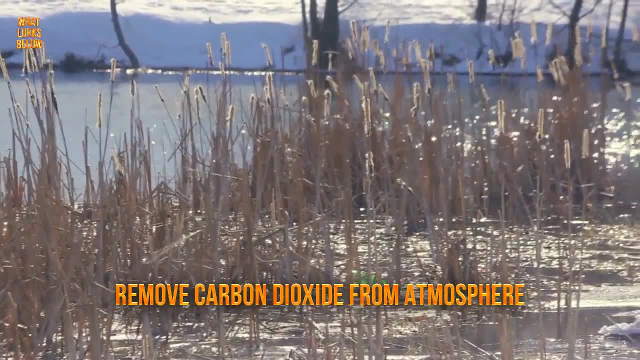 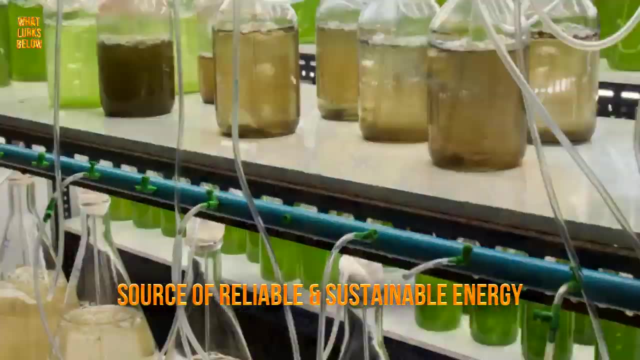 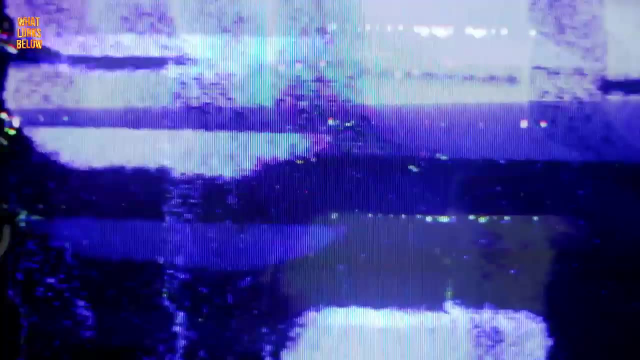 Due to this powerful relationship with the sun's rays, plankton is a proven source of reliable, sustainable energy. Thanks to plankton, we can count on these two natural resources to give our planet the economic upgrade it deserves. Number 1. They wreak havoc in the tide.